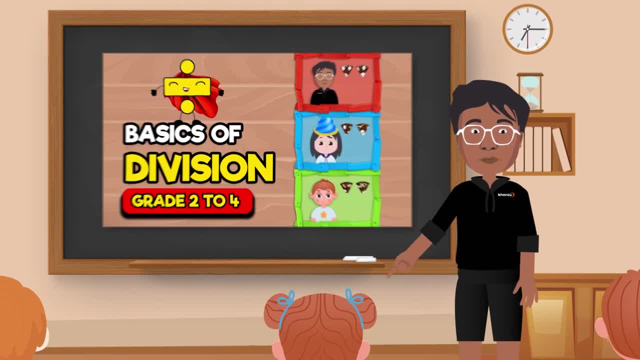 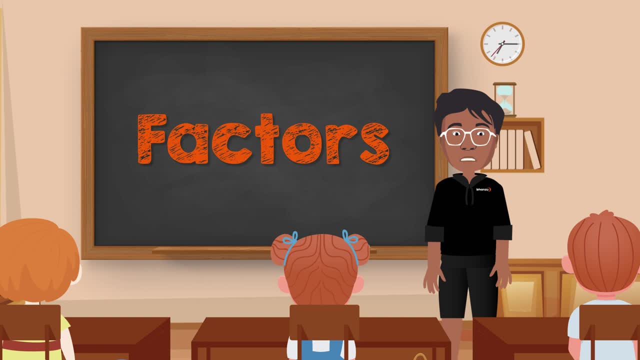 head straight to our Basics of Division video. So, since you all understand, division factors are going to be simple. Factors are numbers that divide a number evenly. For example, the factors of 8 are 1,, 2,, 4,. 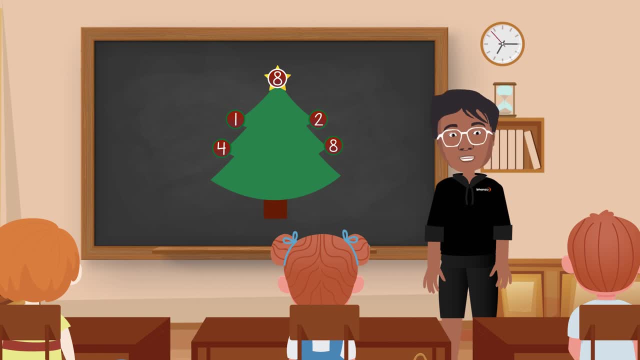 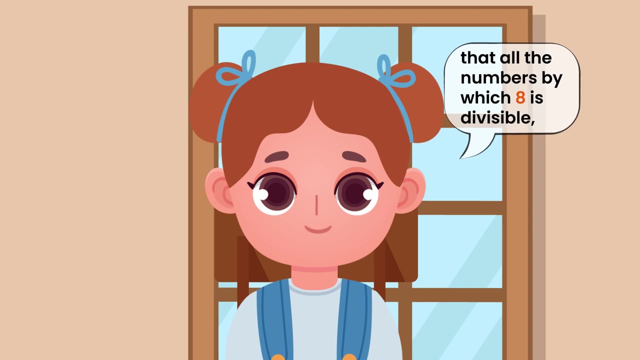 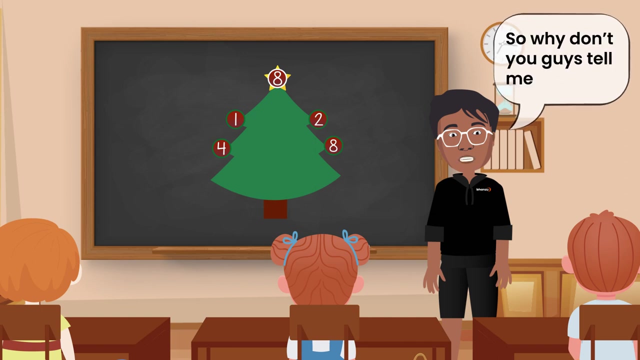 and 8 itself. This means that when we divide 8 by either of these numbers or either of its factors, we are left with no remainder. This means that all the numbers by which 8 is divisible are its factors, right? Yes, Anna, you are absolutely right. So why don't you guys tell me the factors of 12?? Let me try, Hmm. since 12 can be divided by 1,, 2,, 3,, 4, 6, and 12 itself, these 6 numbers are its factors. 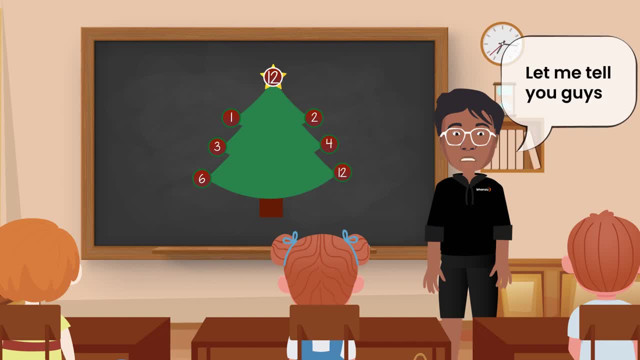 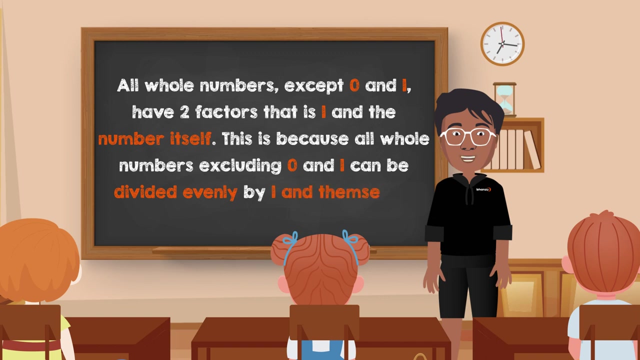 Yes, that's correct, Peter. Let me tell you guys a fun fact about factors. All whole numbers, except 0 and 1, have 2 factors, That is, 1 and the number itself. This is because all whole numbers excluding 0 and 1 can be divided evenly by 1 and themselves. 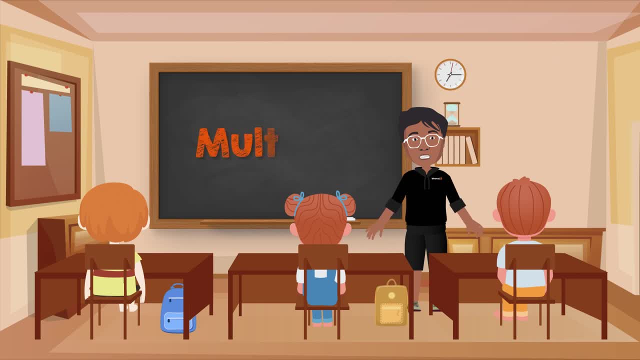 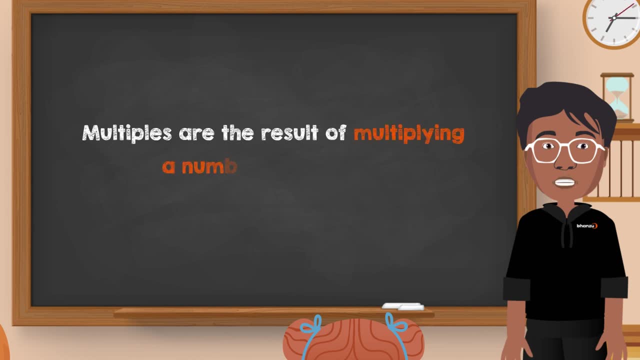 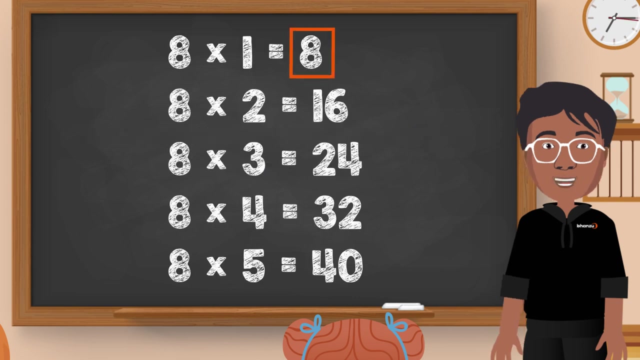 Now moving on to multiples. As the name itself suggests, multiples are the result of multiplying a number, a number, by another. For example, the multiples of 8 are 8 itself, and then 16,, 24,, 32, and so on. 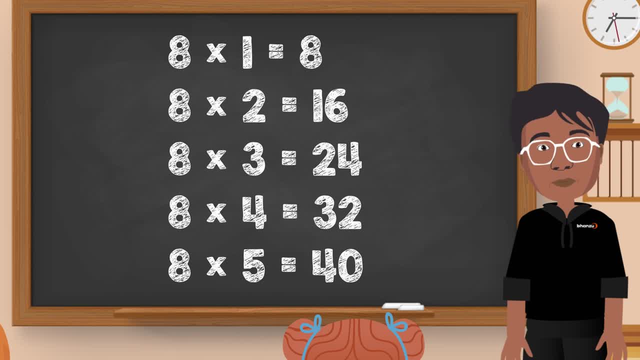 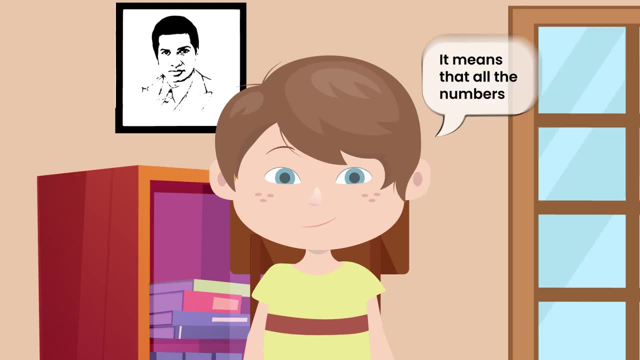 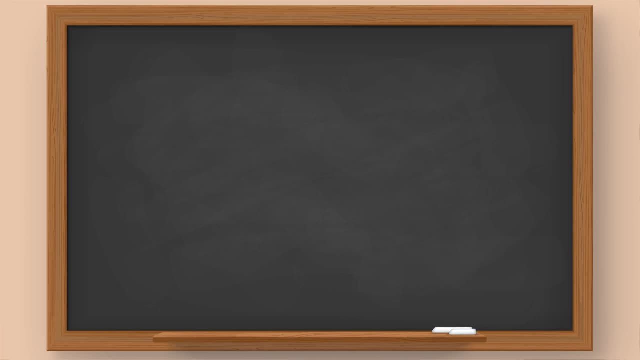 You take any number and multiply it by 8, the product is going to be a multiple of 8.. Easy, right. It means that all the numbers in the table of 8 are the multiples of 8.. Right Like: 8 multiplied by 5 equals to 40.. 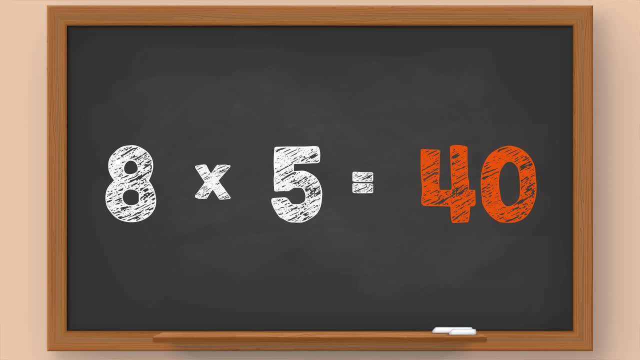 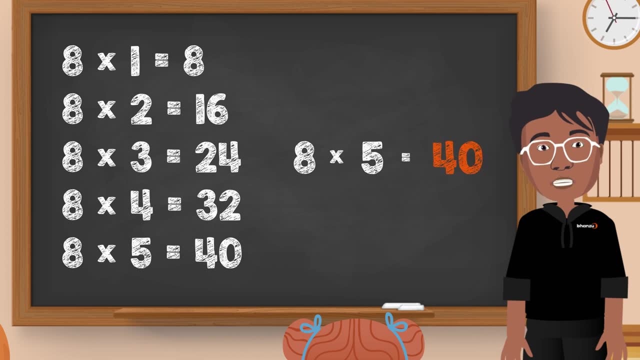 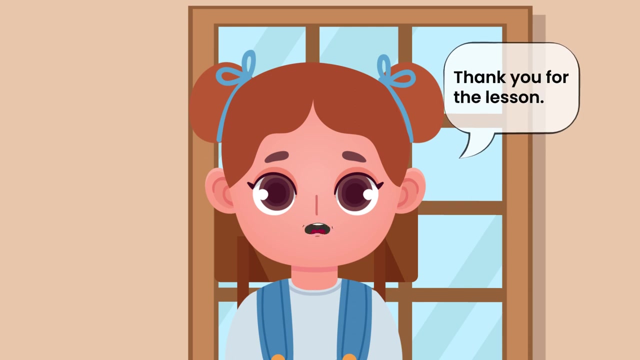 So 40 should be a multiple of 8.. Right, Yes, John, You're right. 40 and all others in the table of 8 will be its multiples. This is super simple, Bhanu. Thank you for the lesson. 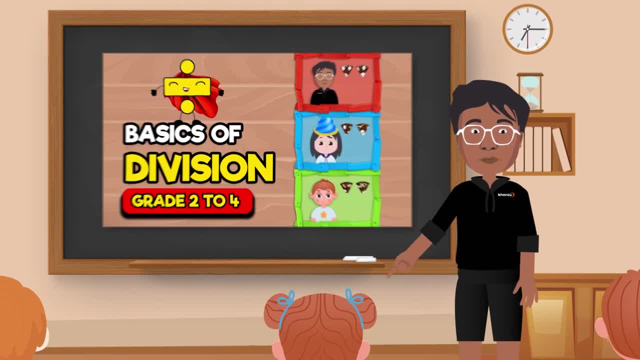 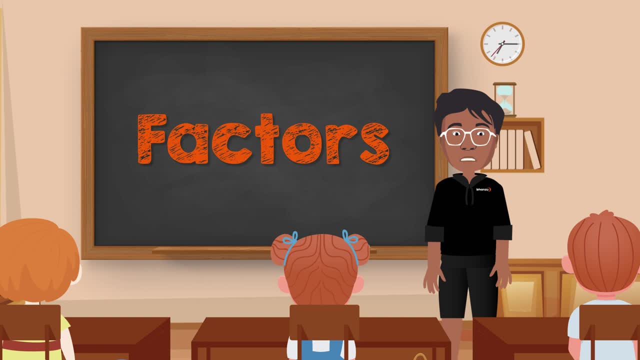 head straight to our Basics of Division video. So, since you all understand, division factors are going to be simple. Factors are numbers that divide a number evenly. For example, the factors of 8 are 1,, 2,, 4,. 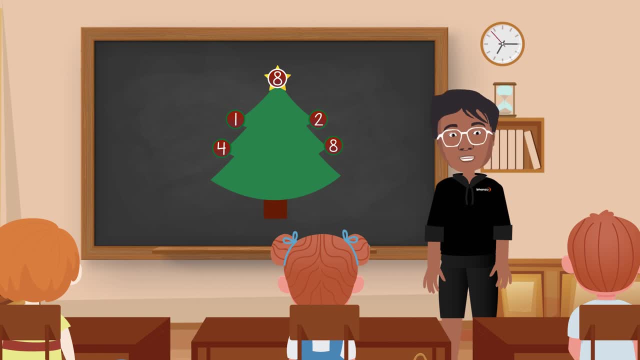 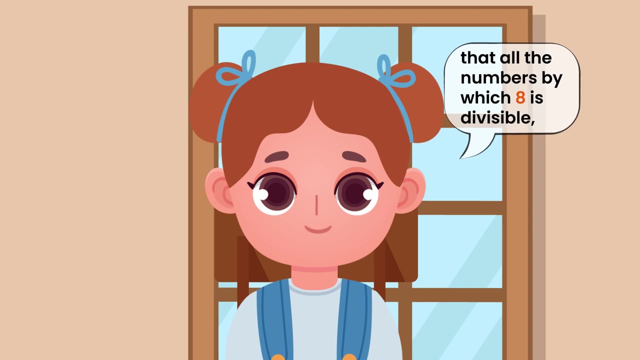 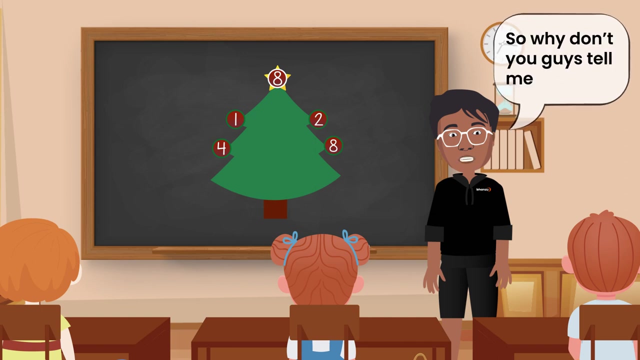 and 8 itself. This means that when we divide 8 by either of these numbers or either of its factors, we are left with no remainder. This means that all the numbers by which 8 is divisible are its factors, right? Yes, Anna, you are absolutely right. So why don't you guys tell me the factors of 12?? Let me try, Hmm. since 12 can be divided by 1,, 2,, 3,, 4, 6, and 12 itself, these 6 numbers are its factors. 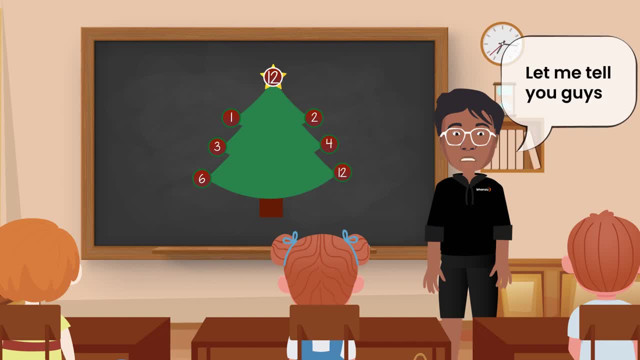 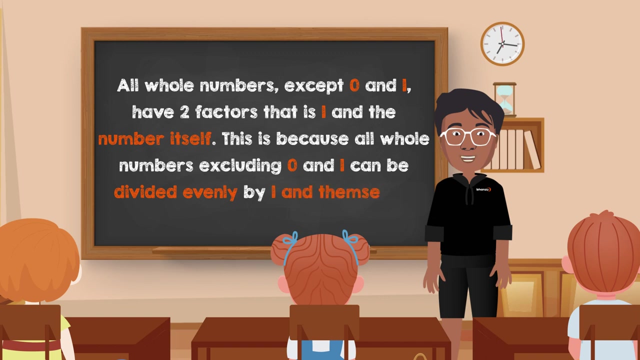 Yes, that's correct, Peter. Let me tell you guys a fun fact about factors. All whole numbers, except 0 and 1, have 2 factors, That is, 1 and the number itself. This is because all whole numbers excluding 0 and 1 can be divided evenly by 1 and themselves. 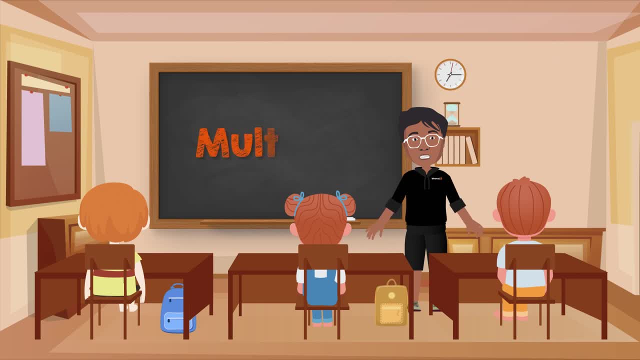 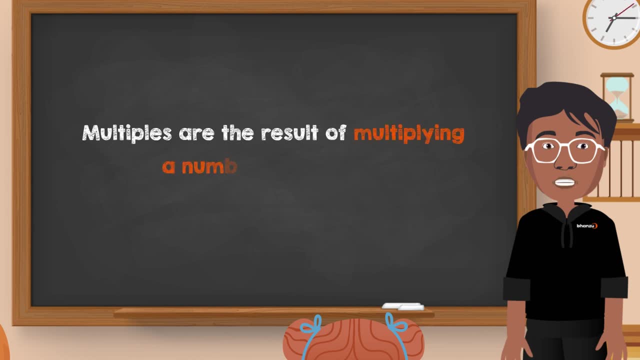 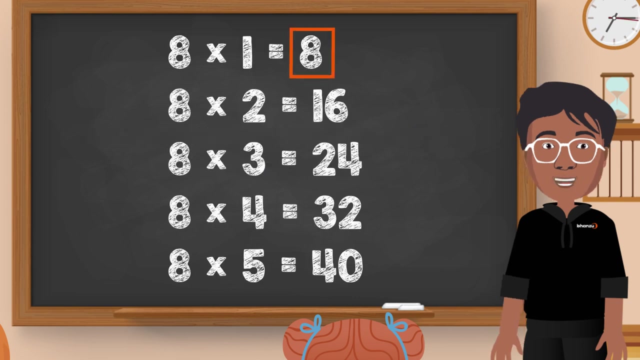 Now moving on to multiples. As the name itself suggests, multiples are the result of multiplying a number, a number, by another. For example, the multiples of 8 are 8 itself, and then 16,, 24,, 32, and so on. 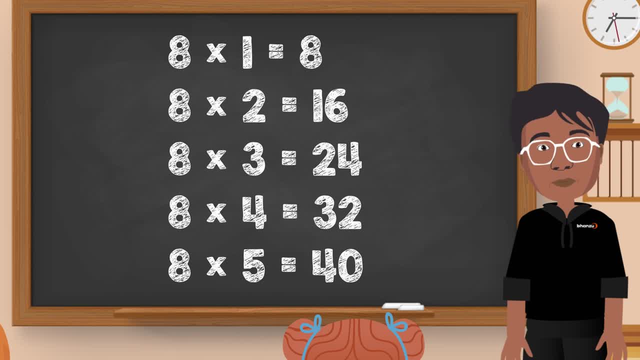 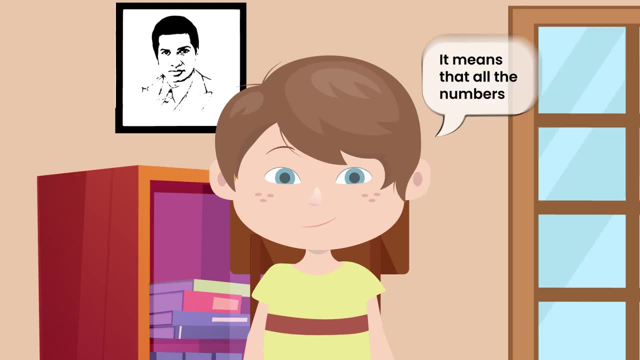 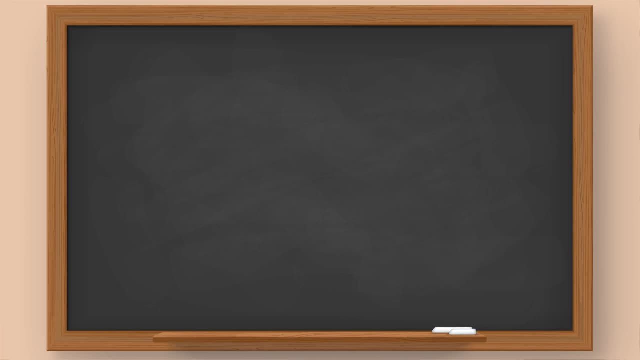 You take any number and multiply it by 8, the product is going to be a multiple of 8.. Easy, right. It means that all the numbers in the table of 8 are the multiples of 8.. Right Like: 8 multiplied by 5 equals to 40.. 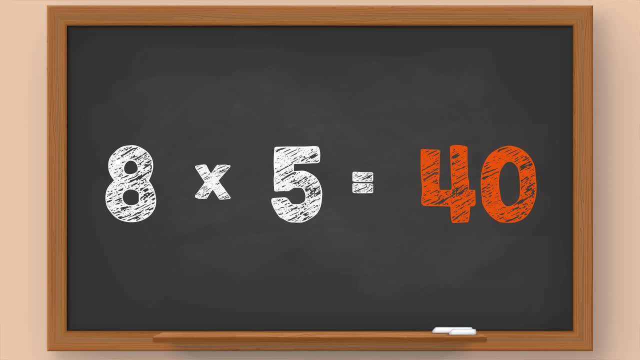 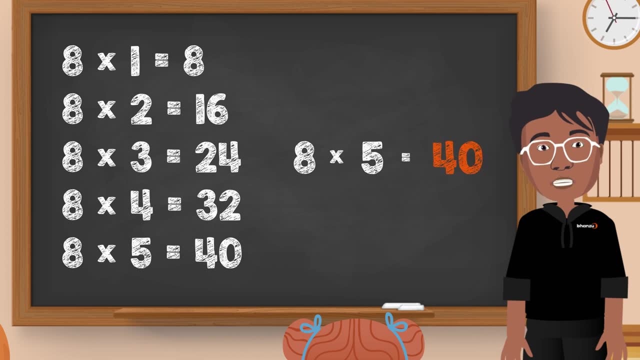 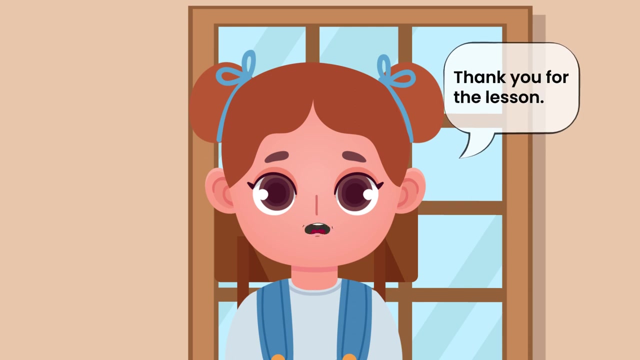 So 40 should be a multiple of 8.. Right, Yes, John, You're right. 40 and all others in the table of 8 will be its multiples. This is super simple, Bhanu. Thank you for the lesson.